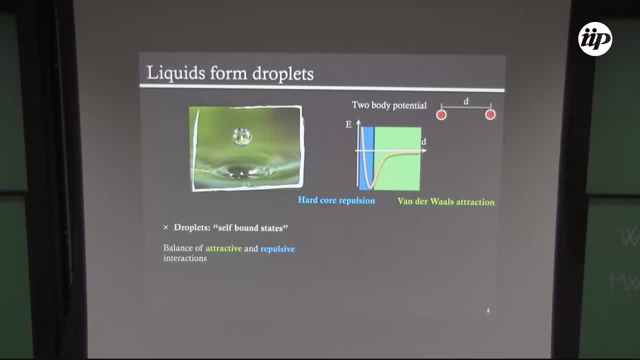 but, however, at short distances we have this hard core repulsion. So, in general, liquids, therefore, okay. so in general, liquids, therefore, are dense systems, because we need some length scale where these two terms they can balance, And that's why liquids are complex system to model And, on top of that, one of the problems of 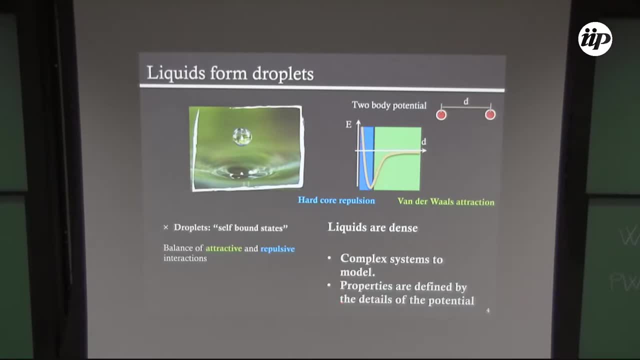 these liquids is fully defined by the details of the process potential. therefore, I need to know all the details of the potential in order to obtain the properties, in order to describe my liquid in a better way. so the question that I wanted to address at ICFO is like: I'm sorry that this is. 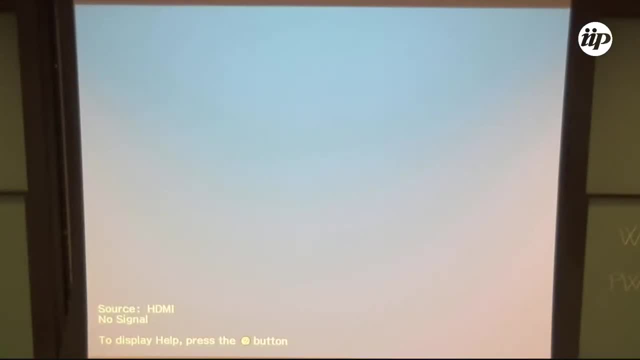 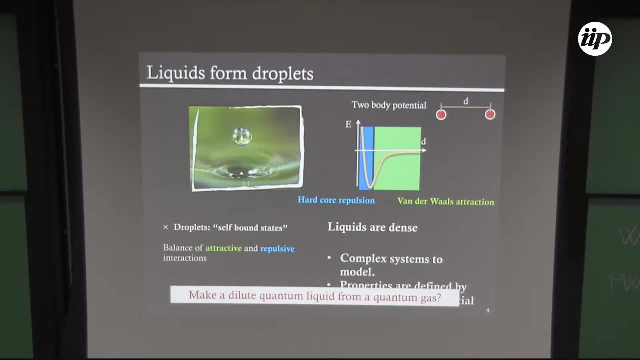 not working. okay, the question that we wanted to address at ICFO is like: okay, can we make a dilute quantum liquid where we can overcome all these problems I just mentioned before? and of course, I don't have to explain to you that quantum gases are really good systems to overcome these dense systems and 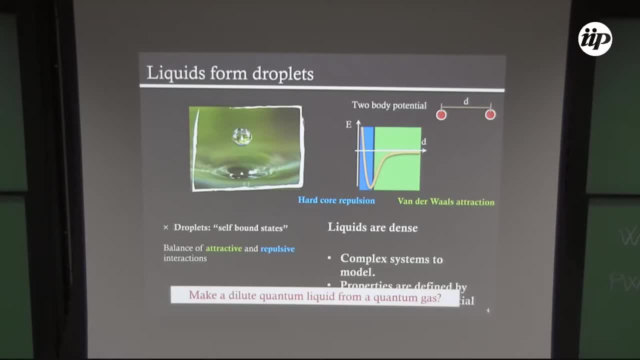 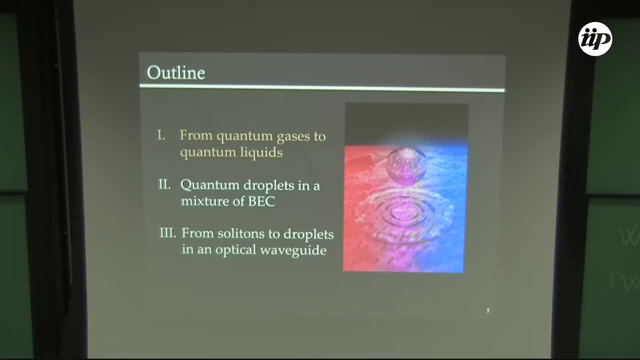 also to define it with just single parameters, so called, for example, the scattering length. so with this I come to the outline of my talk. so first I will explain, like how, the theory, how to go from quantum gases to these quantum liquids. I will explain the experiment that we have perform at ICFO. 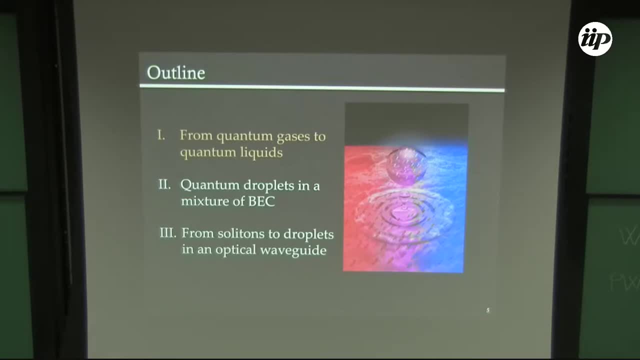 so. So we can observe these quantum droplets in the mixture of boson instant condensates. And finally, if I have time, I will also explain the difference between solitons and droplets, because in fact these two systems are cell-bound states, or at least bright solitons are well-known. 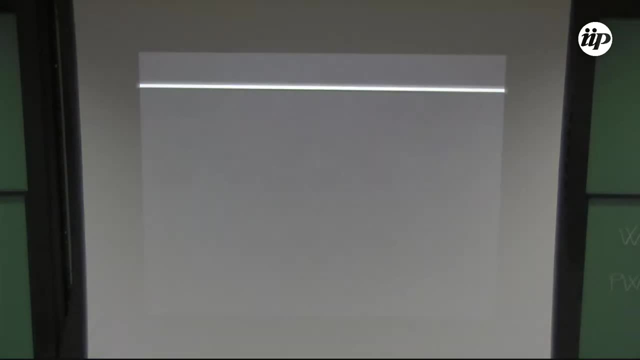 cell-bound states that exist in the community. So, as I explained before, how can we create a liquid? using a gas or using a boson instant condensate? So first we need attractive interactions to hold the system together and in fact, in 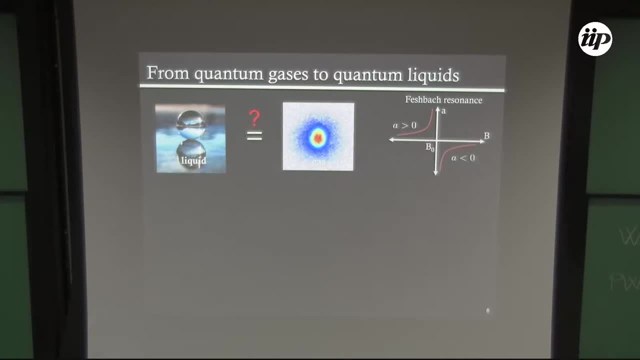 VEC. this is pretty simple because we can just use fresh back resonances. So therefore I can tune the interactions in my condensate to be attractive, but this will be the mean field energy associated to my boson instant condensate. 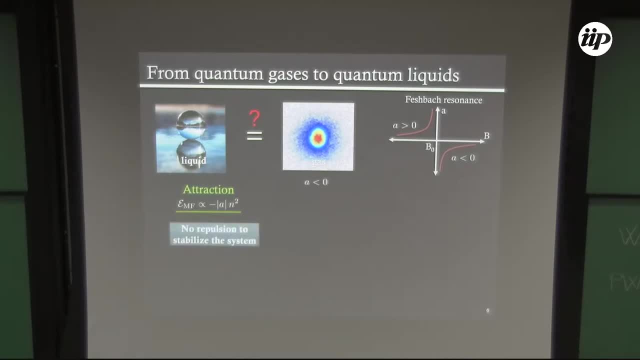 That depends on the scattering density square, But however, at this length scale, there is no repulsion that can stabilize the system, And what will happen is that my VEC will collapse And, in fact, This is something that we will talk about during this session. 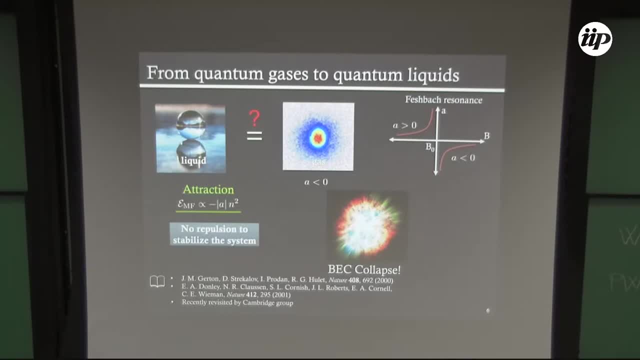 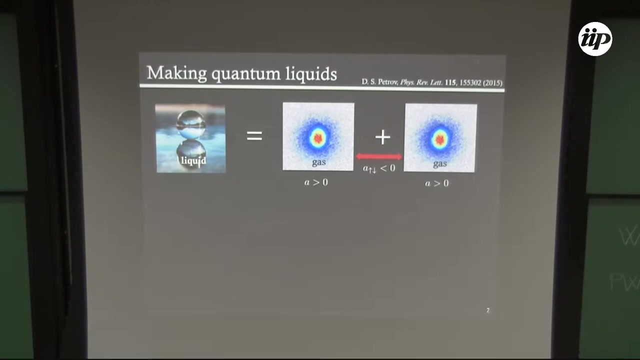 something that was studied during the early times of VECs, where this VEC of the collapse was revisited in these different papers. But this is the end of the story. So, Dima Petrov in 2015, he realized that okay, maybe, instead of using just one single component, boson instant. 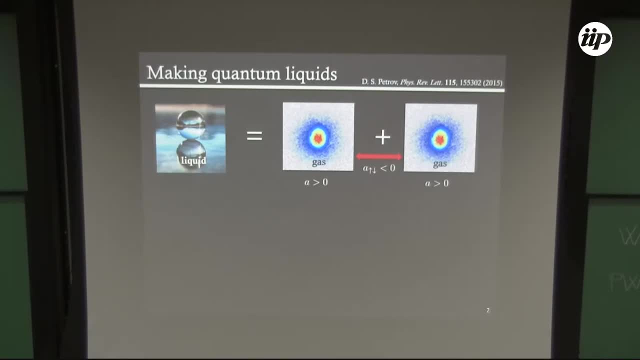 condensate. we can use two component boson, instant condensate, which has repulsive interactions- each condensate but attractive interactions between them. In this system I can define this concept or this delta A. that will depend on the difference between the inter- and 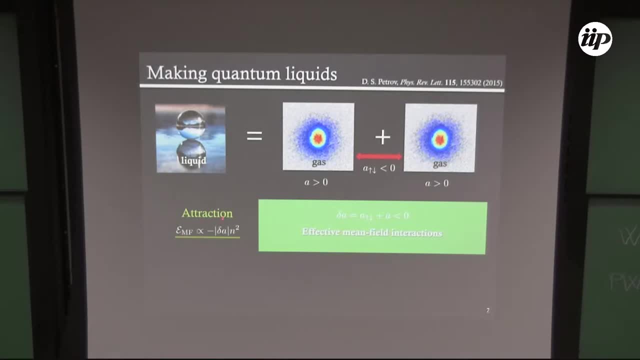 interspecies interaction. I can also define my mean field, energy, as I did for the single component boson: instant condensate. This will depend on delta A and N squared. But what is really interesting is that in these two component condensate we have some extra repulsion. 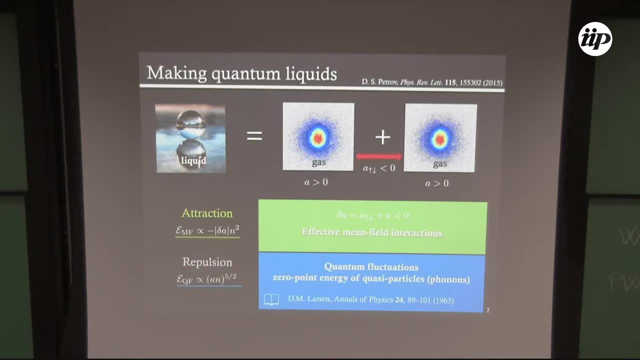 that becomes important. that comes from quantum fluctuations or beyond mean field terms. This repulsion depends on the scattering length A, and it has an scaling on A. So in this case I can find a situation where I can tune my delta A close to zero, or maybe. 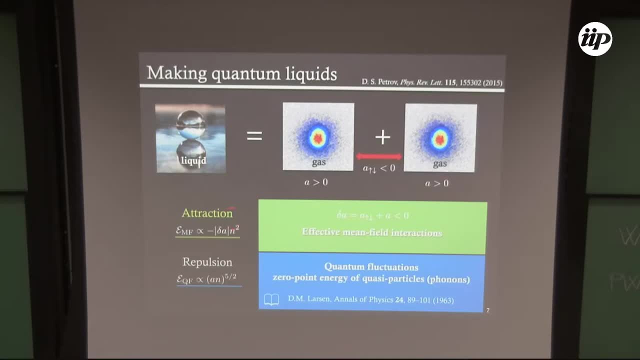 even zero and kill. therefore this mean field energy, or make it really small and comparable to the quantum fluctuations, or this repulsion extra term that can stabilize my system. So therefore, for a given delta A, I can find an equilibrium density that 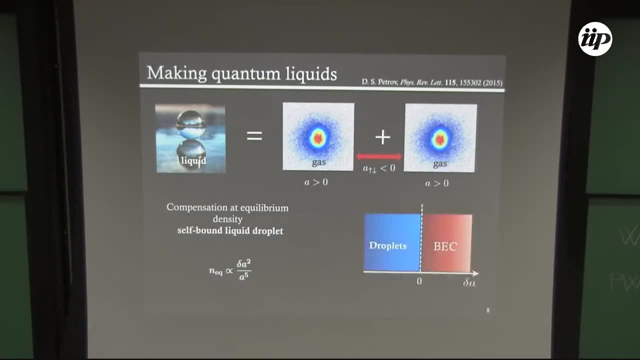 will depend on just only interactions And therefore this will be more relevant to the interspecies interaction. So in this case I can find a phase diagram. For delta A positive, I will have a boson instant condensate, but for delta A negative, I could find an equilibrium density that will stabilize. 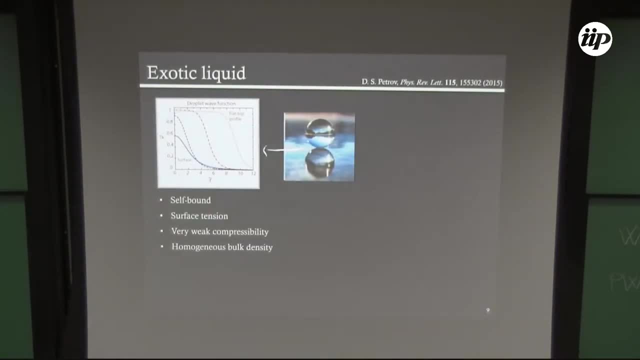 my system. This is a very exotic liquid because I mean first will be self-bound, using just two component boson, instant condensates. It will have some surface tension, It will have some very weak compressibility And what is an interesting property is that it will have some homogeneous. 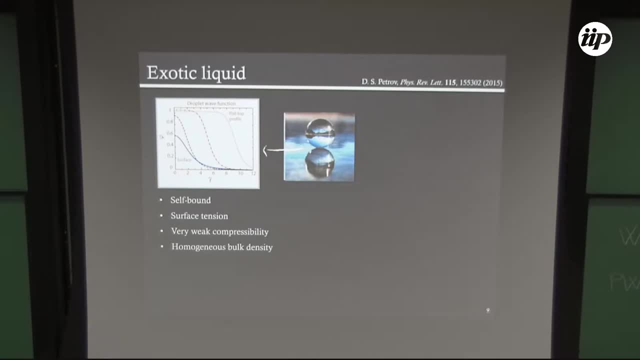 bulk density because, as I explained before, the equilibrium density just depends on the, just depends on the interactions. So I mean, once you have the right interactions, if you put more and more atoms, the density has to be constant. So therefore, this is the wave. 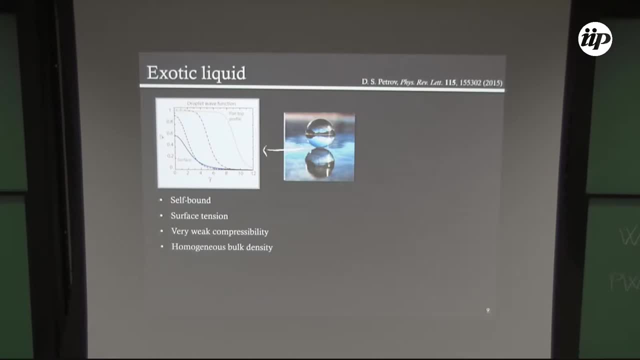 function or the profile that I expect to see. So for a given equilibrium density, I will have a flat-top density profile and this will be part of the surface of our droplets. If I put more atoms, just this wave function will increase. 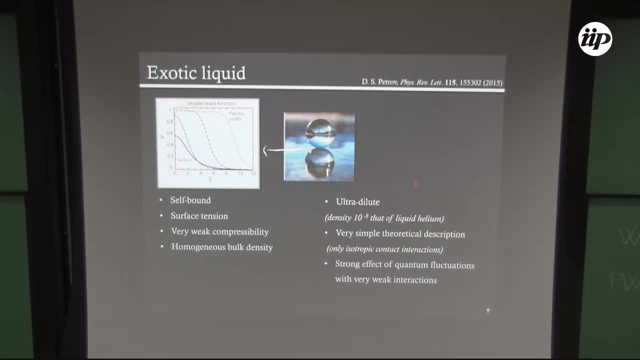 For the experimental parameters that we use in our lab. so this is a really ultra-dilute liquid that, in fact, is like eight orders of magnitude more dilute than any other liquid in nature. And the advantage is that it has a very simple theoretical description, because 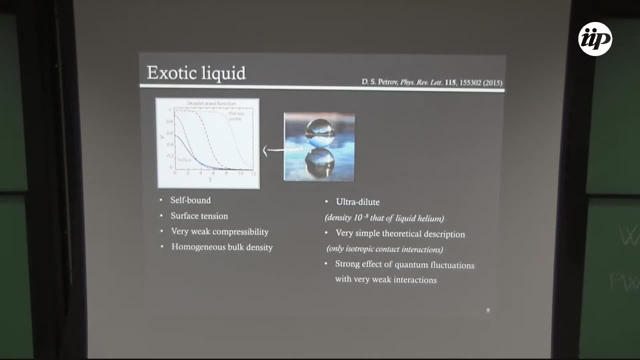 it's made only of isotropic contact interactions or the scattering. And the advantage or something that is really nice from these droplets- if they exist, is that the appearance is just due to the strong effect of quantum fluctuations, And this is what I will show If you want to have more details about the properties. 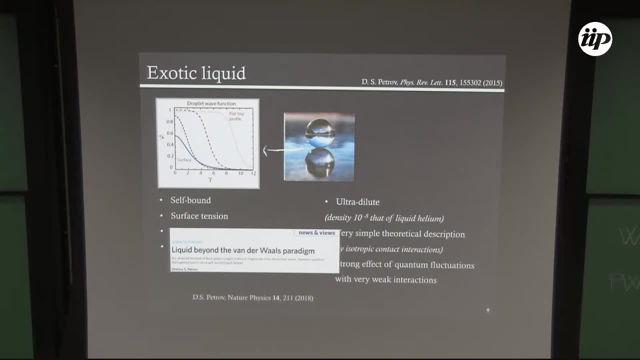 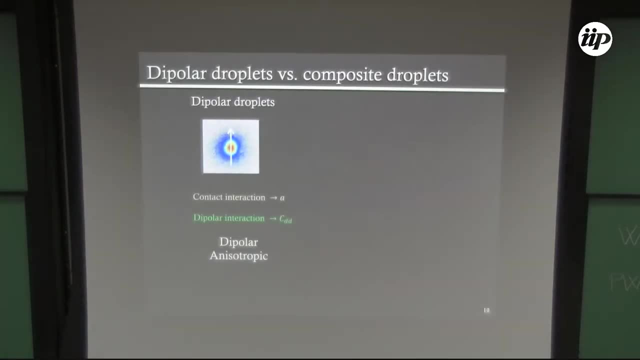 of these liquids. so there is a really nice review from Dima Petrov where he explains how these liquids go beyond the Van der Waals paradigm. Of course, this is not the only system that droplets could exist. They can also exist. 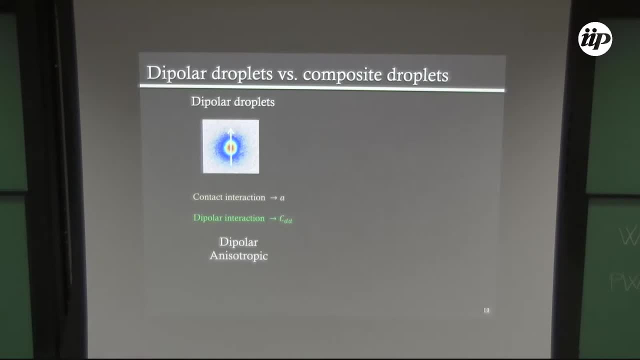 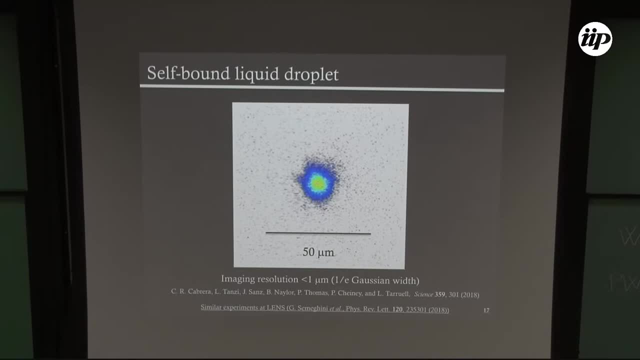 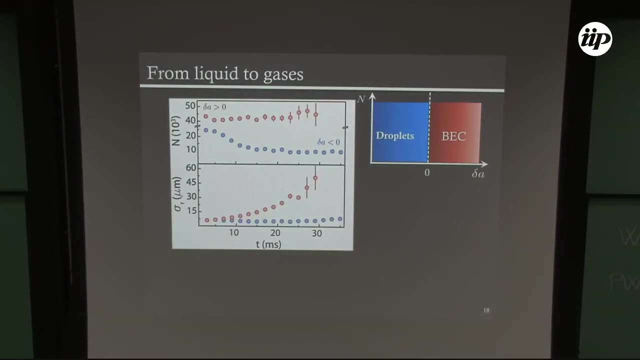 group of Tillman Pfau and also Francesca Ferlaino have shown- Then we have a second now- are complementary to the results that also in LENS have been working. Okay, so now let's analyze a bit data that we observed in the lab. so the red points: 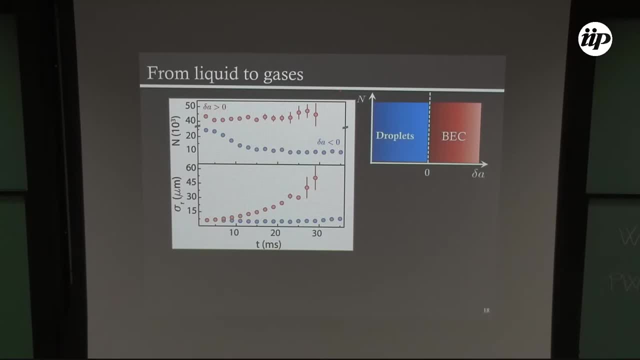 I will show. it's the gas, a delta A positive system, and the blue points is delta A negative. so it's the droplet phase or the liquid phase First. if we observe in data number or the size as well, the size we can see in time. 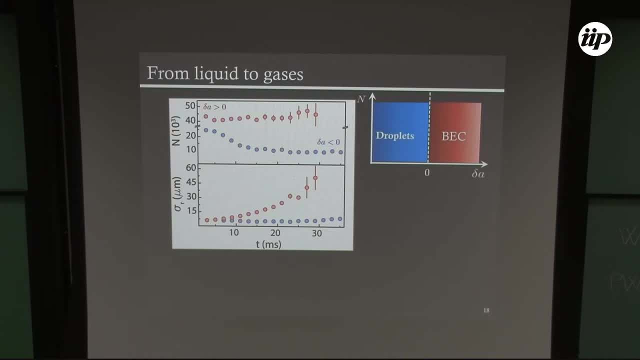 that it just expands as a normal gas, but we see that in the case of a liquid it just remains cell bound. What we observe also as well is that the atom number decay in the case of the droplet phase, while in the gas phase it just remains constant, and this we attribute, this decaying atom number. 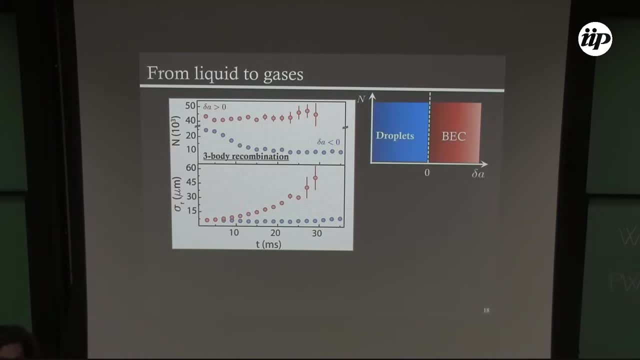 to three-body recombination, And this is because our droplet remains cell bound for a long time, so the density is pretty constant. so that's why we observe these losses, up to a point where this three-body recombination is not more important. 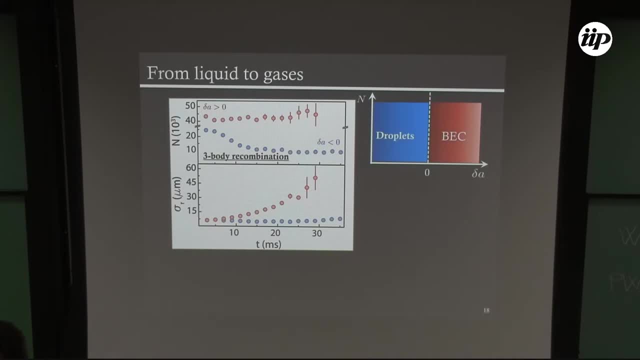 Okay In the case of the gas, because it just expands really fast, so it becomes really dilute, and then that's why we don't observe this effect. What is interesting is that if we zoom this part from here, we will see that, yes, the 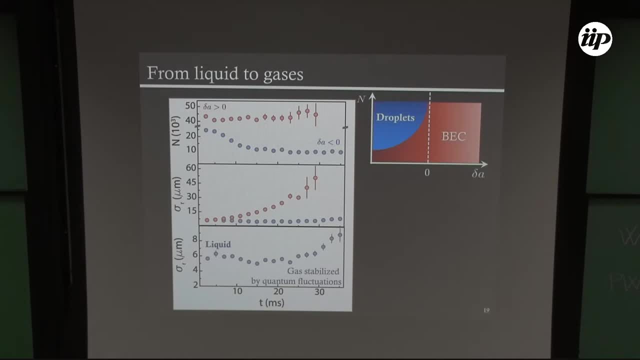 liquid phase. it's constant. the size is constant just for tens of milliseconds. but then it grows up. And this is because before what I present is, I was just taking into account the mean field, energy and the Li-Juan-Zhang. but also we know that we have quantum pressure. but 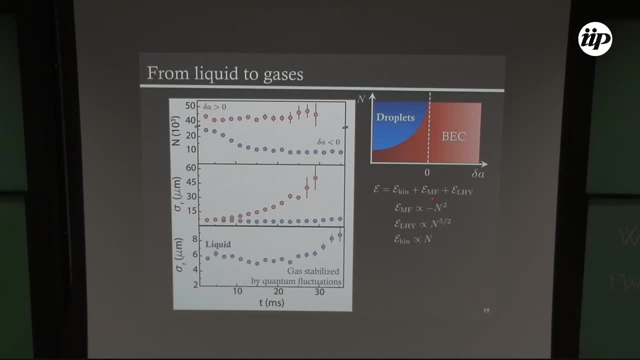 in this case, for example, we have quantum pressure. So for low atom number, the scaling that depends on n becomes important, and actually this is what dissociates our droplets. So what we are observing here is that for low atom number, the kinetic energy is actually 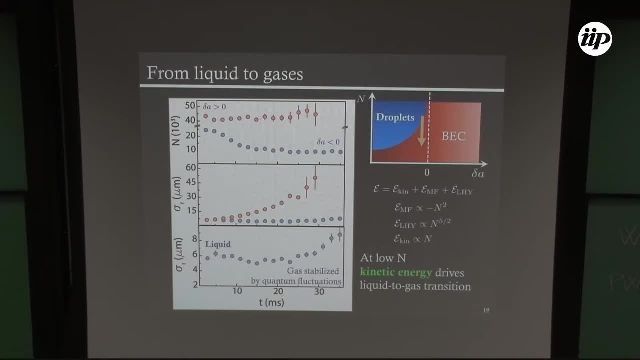 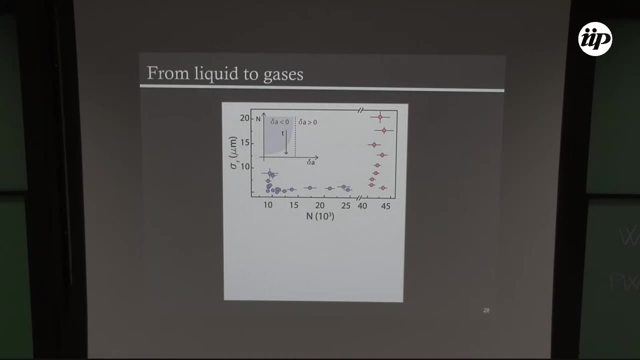 driving a liquid to gas phase transition in the system. We have plotted this in the size as a function of atom number. So what we observe is like: for a given atom number the size remains constant, but then for a critical atom number this size diverges. 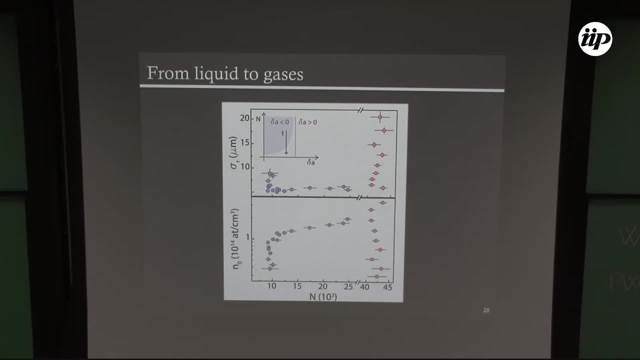 And this is where the transition occurs in the system. We have as well observed the same if we plot in terms of density, where the density remains constant and then just behaves exactly like a gas, as I showed here in the red points. 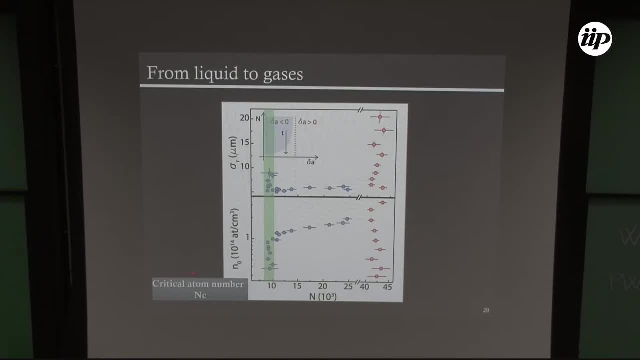 So, using these observables, we can extract the critical atom number, or we can extract where this transition occurs, as a function of the atom number and also as a function of the interaction strength. This is what we have observed, Thank you. So this is what we have done. 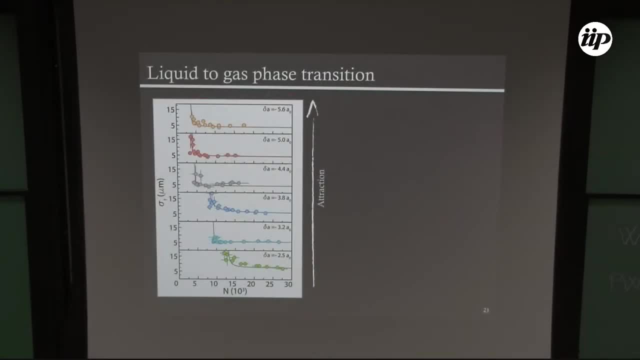 And then, as I showed here, depending on this delta A, as we can observe, when this delta A becomes stronger, so we need less and less atoms to remain this system, cell bound. That is more or less what we observed here in this phase diagram. 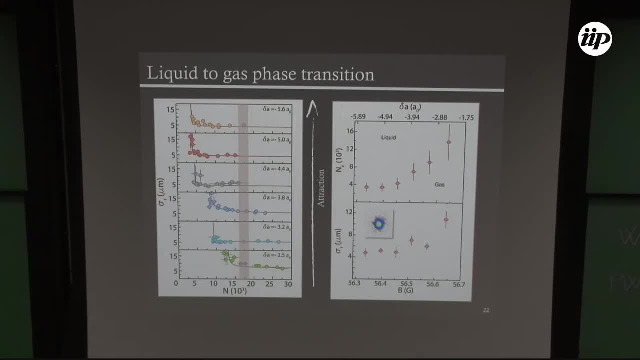 And then we have made these kind of plots for different interaction strength, and this is what I showed here. This will be the line for the phase transition: Above is the liquid, Below is the gas. And then we have also plot for a given atom number, the size that we can resolve in our 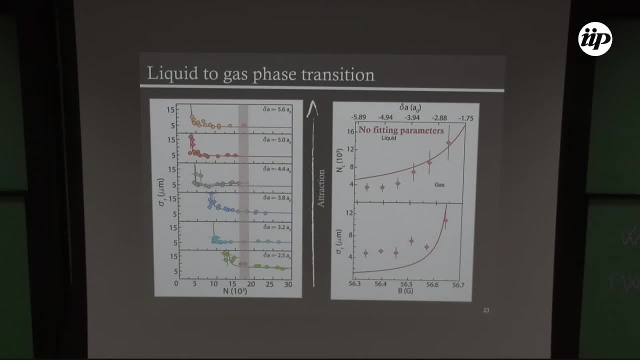 imaging system And we have compared this with the theory and adding this Liguang-Zhang correction, And what is interesting is that, OK, using no fitting parameters, this theory fits, I would say, quite well with the points. And then what is interesting to remark is that this system is a very sensitive test. 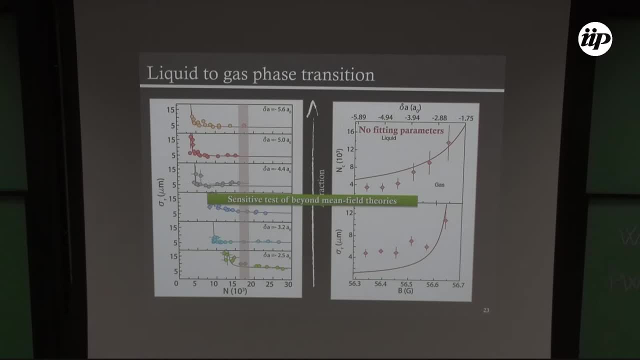 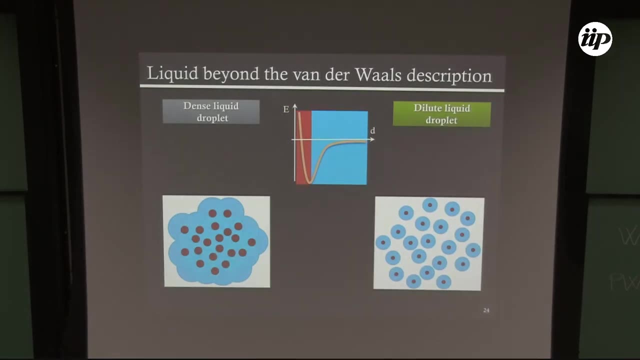 of beyond-measurable field theories, because the existence of this quantum liquid droplet is due to this Liguang-Zhang term, And just to give you a flavor why these liquids are nice. OK, this is the two-body potential I present before. 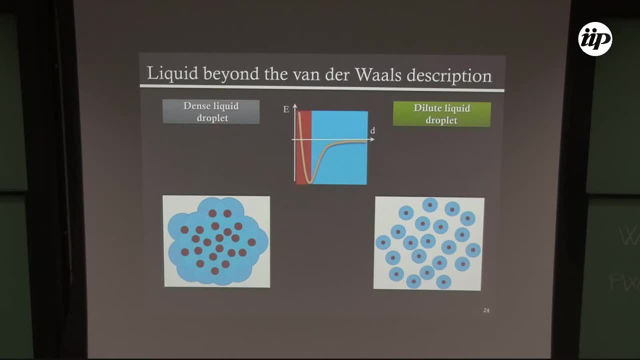 So we have the attractive part and the repulsive core And in the case of our liquids- basically liquids- they look like this: I mean we have the core, but this is this red part, and then we have the blue. that 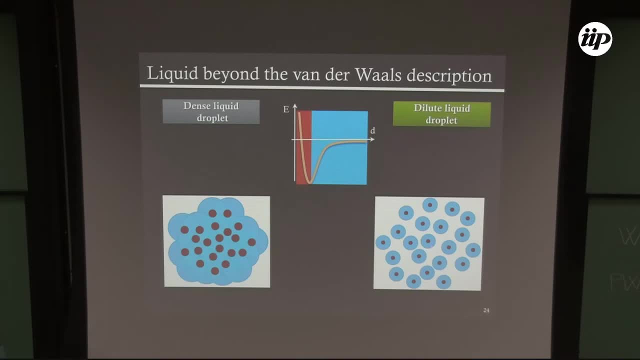 is the attractive one, and they are really dense and they are really close together. In the case of diluted liquid they are very dense. So what happens is that this potential it doesn't even play a role, and the atoms, they are really really far apart from each other, but still they want and remain together. 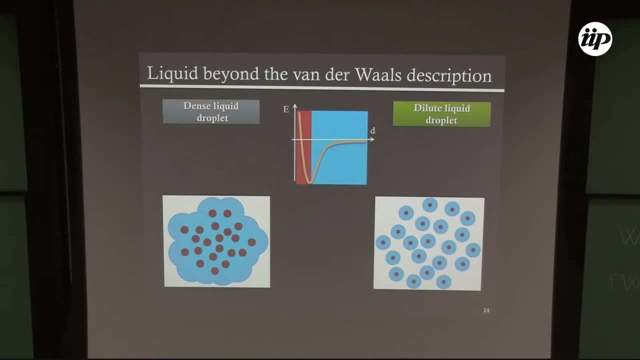 So this is the picture that you should take from these ultradilute liquids. but really the atoms are so far apart, but still they remain together and they have some surface tension and properties of liquid. And again I mean I have this nice picture. 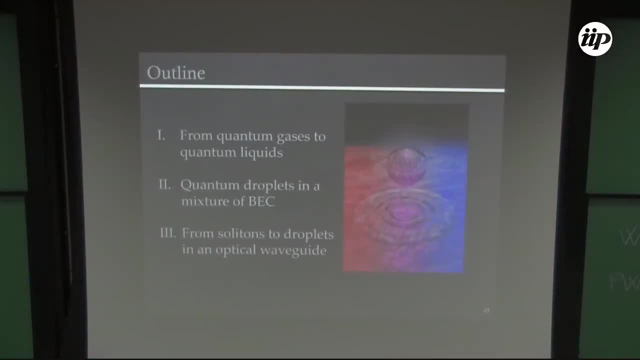 Review of liquids beyond the Van der Waals paradigm. And I don't think, yes, OK. so now I will explain. OK, what I have shown up to now is just these quantum droplets that are cell-bound states, but however bright solitons are also, 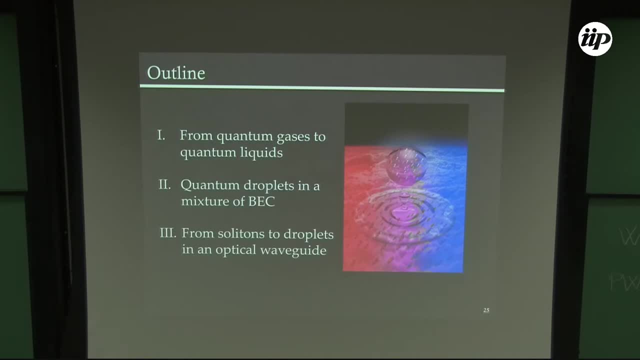 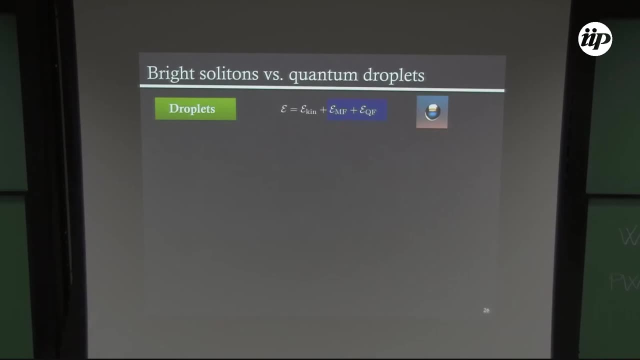 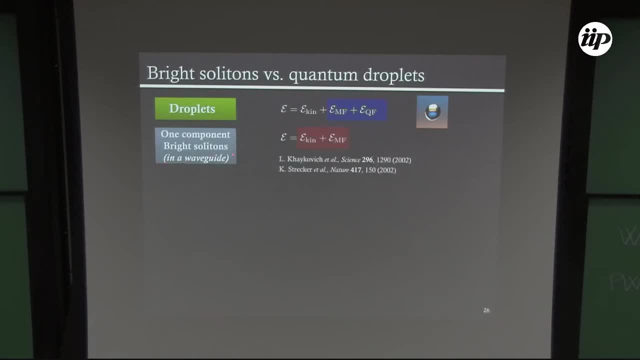 and the quantum fluctuation term. However, one component, bright solitons. they appear due to the balance of the quantum pressure and the mean field energy In our system. if we place a voce-voce mixture in an optical waveguide, what will happen? 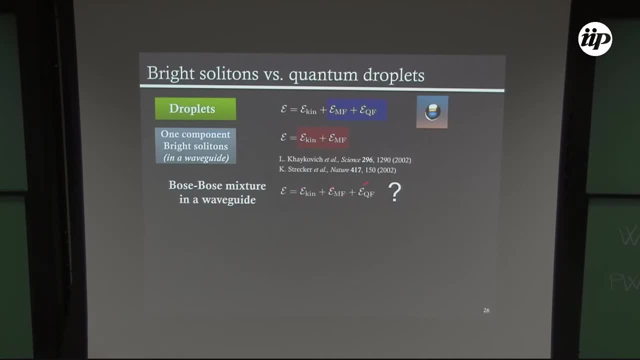 is that we will have these three terms: the kinetic, the mean field and the quantum fluctuation part and both at some point the effect of the three will interplay. So what I will expect to see is either a transition or a crossover between the two systems, because 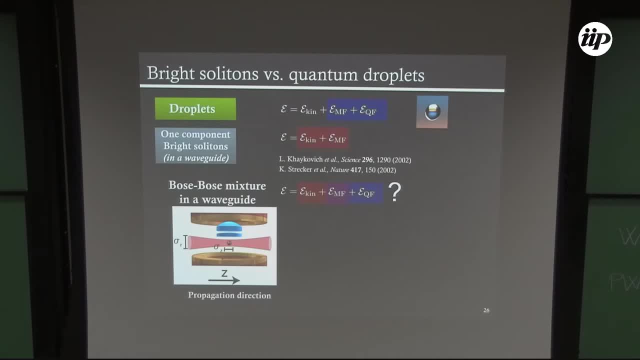 the three energy terms. they play an important role. So what we have done is the following experiment: So we have played our voce-voce mixture in the same magnetic window and using the same imaging technique that I explained before in an optical waveguide. 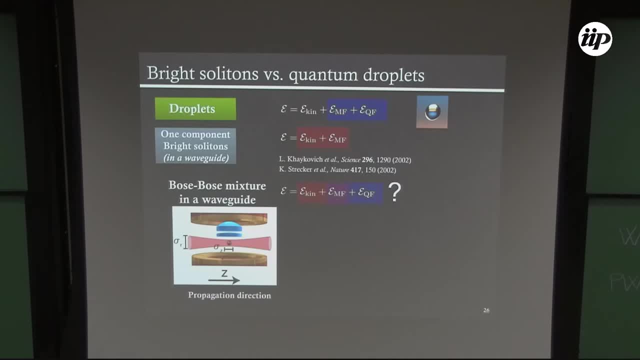 Here I refer to quasi-one-dimensional physics, in the sense that we constrain just the transversal degrees of freedom, but the longitudinal degree of freedom, the longitudinal degree of freedom, the degree of freedom is free to expand, and this is what we have observed. 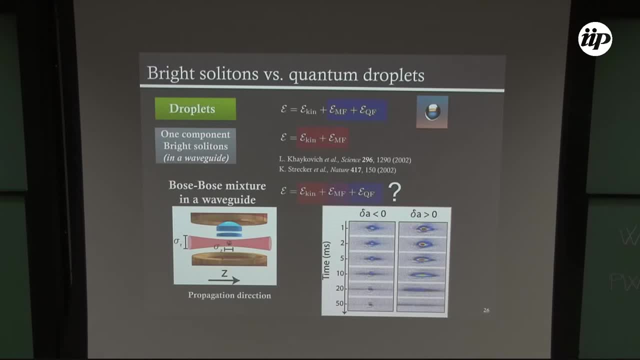 For delta-A positive. so my system just expands as a normal voce-instant condensate, but however, for delta-A negative we observe a self-bound state. So now the question is like: is this a soliton or is it a quantum droplet? 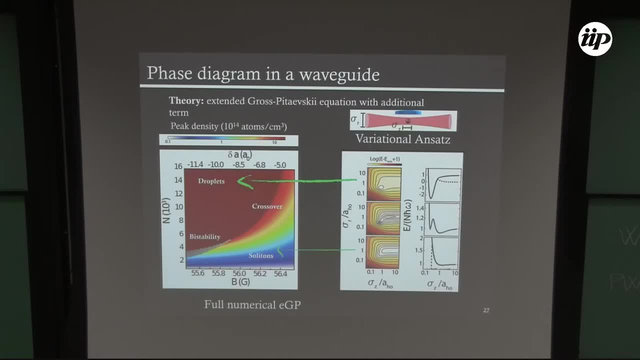 We have performed the theory, We have used the Grosbe-Typsky equation and with this additional Ligman-Jean term, and this is what we have observed- We have done it numerically. We have done it numerically and also using a variational ansatz. 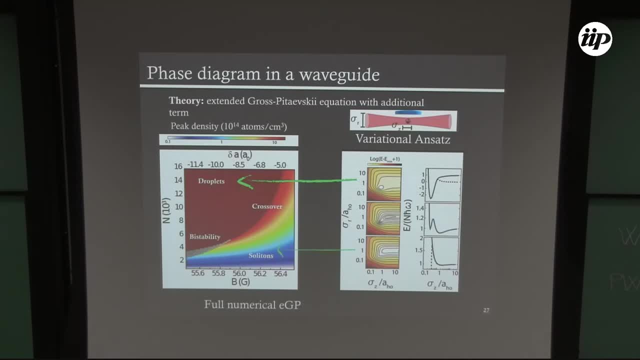 So what you observe here is the magnetic field, or interaction at strength as a function of a factor number. The color plot is the density, and what we observe is that we have low-density solutions, that in fact, using the variational ansatz, we observe that the size of these solutions 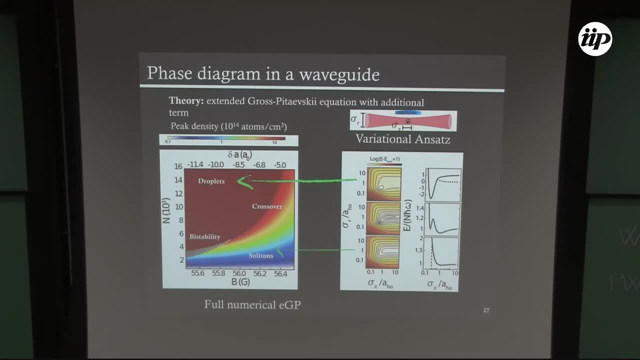 are in the order of the harmonic oscillator length. so therefore these we call that are solitons. We observe as well that we have high-density solutions and in our variational ansatz we observe that the size of these high-density solutions are in the order of the harmonic 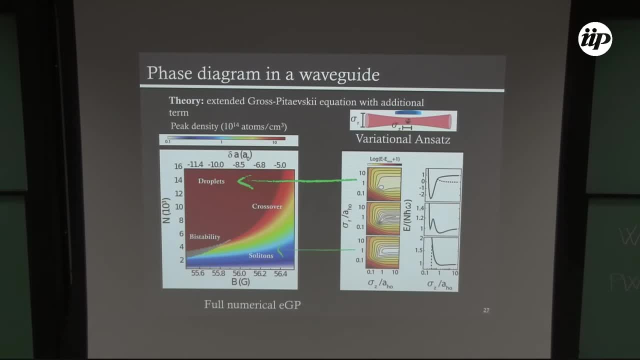 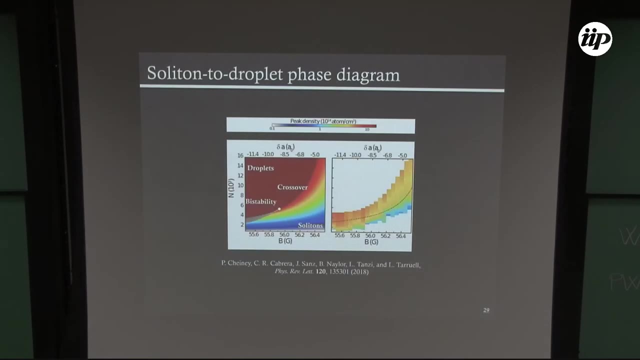 oscillator length. So this is what we identify as droplets, And what is interesting is that, in fact, we observe a bi-stability where we have the two minimas and metastable states, and also a critical point, as I showed here. 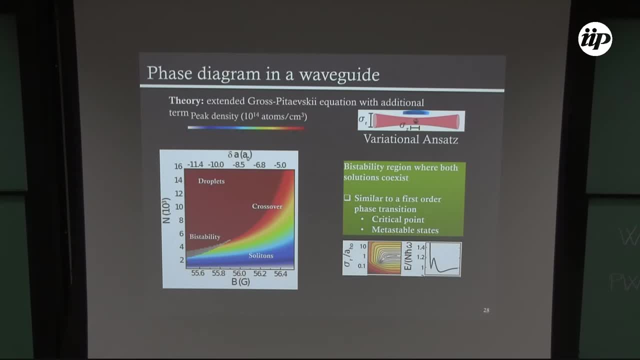 So this is interesting because this bi-stability region is similar- like to have a first order phrase transition. We observe that we have a critical point. We observe that we have also metastable states. We observe that we have a critical point. 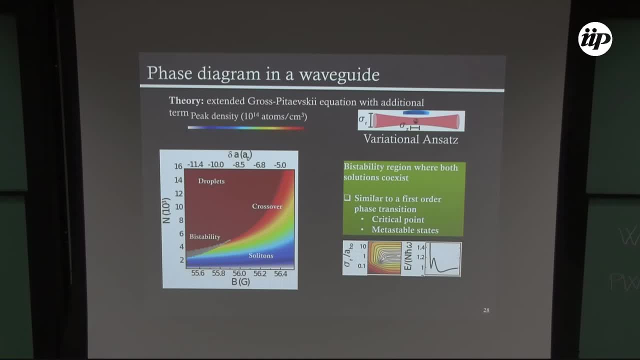 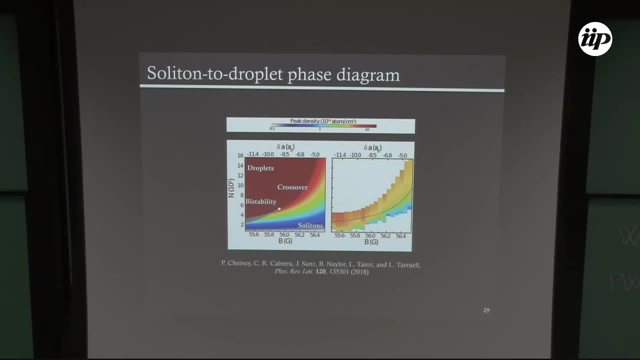 We observe that we have also metastable states. We observe that we have also metastable states And how these two minimas, they can appear or disappear in this bi-stability. So we have explored this experimentally, because what I have before is just a theory. 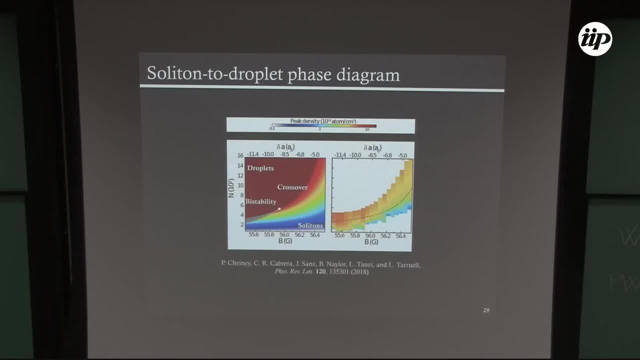 We have measured the density of this cell-bound state as a function of atom number and interaction strength, as you can see here. I mean we have quite well agreement with the densities that we have expected to observe in the theory. What is interesting is this dashed line that I show here. 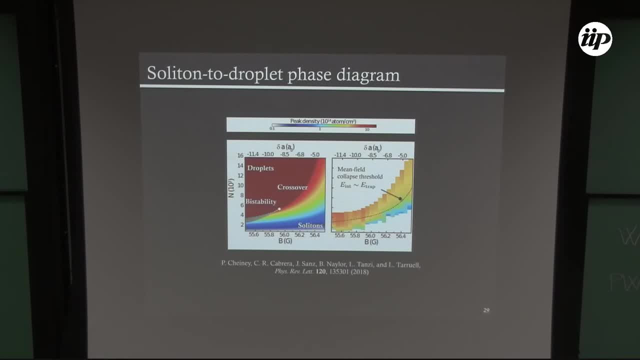 This is the mean field collapse threshold. This is the mean field collapse threshold. This is the mean field collapse threshold where I expect that my solitons should just collapse And we see that we can form cell-bound state. that goes beyond this mean field collapse. 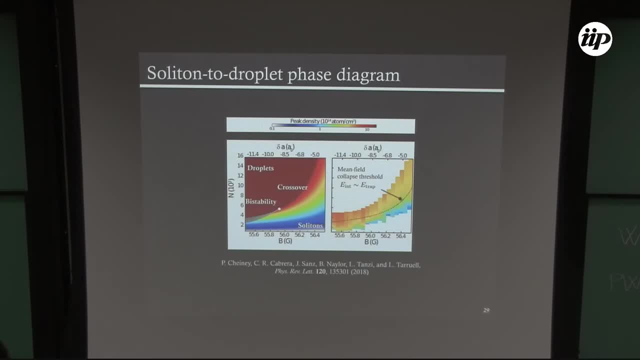 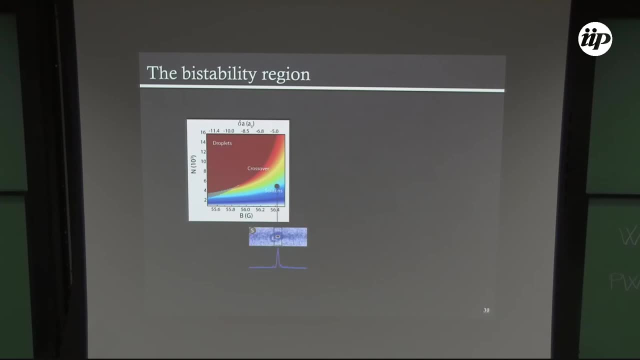 threshold, which means that we have this extra term that actually is the Ligandian term. that is playing a role And that's why our system is not collapsing. We have as well established this bi-stability experimentally, So we have prepared solitons here. 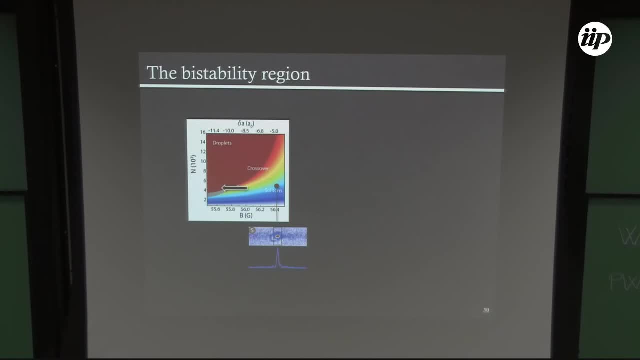 And then we have rammed down our magnetic field to cross the bi-stability and see what occurs. what we observe is the following: we observe fragmentation of the system, and the way we explain this fragmentation is because this is obtained using our variational ansatz. 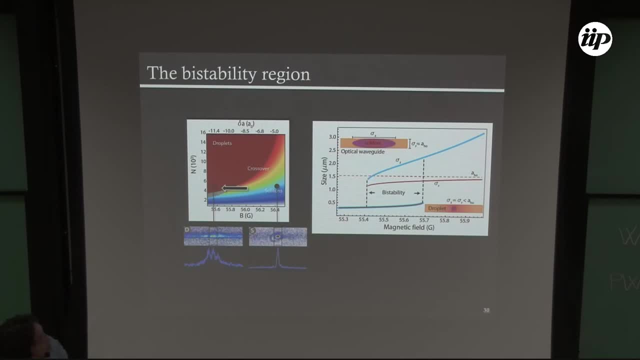 so this blue and red line are the size of our soliton, meaning this regime. and then, when we cross the stability, what happens is that we have a discontinuity on the density. therefore, we go from this side to this side. my system cannot adapt to this discontinuity. 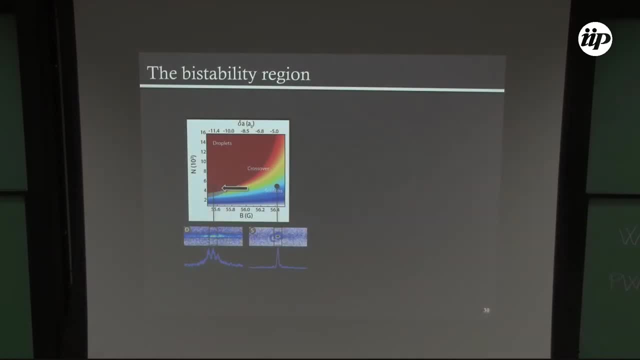 in density. that's why it fragments. We have measured the point where this happens and this is the plot I show here. we measure the atom number in this small crop that I show here in these pictures and we just see how this atom number evolves as a function of the interaction strength. and then we take 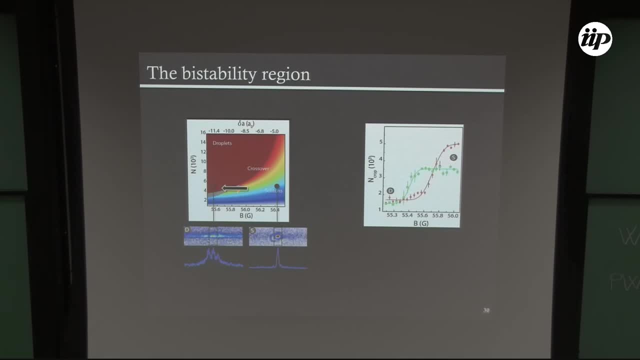 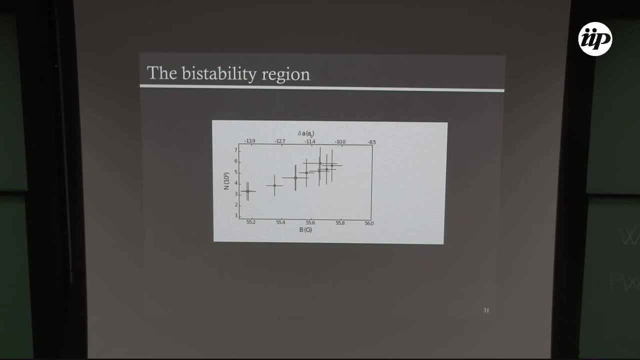 as a middle point, we see that, depending on the initial atom number- so depending where I start here- this fragmentation occurs in different points. So these are the experimental points that we have measured and in fact these lines are the ones that we measure. 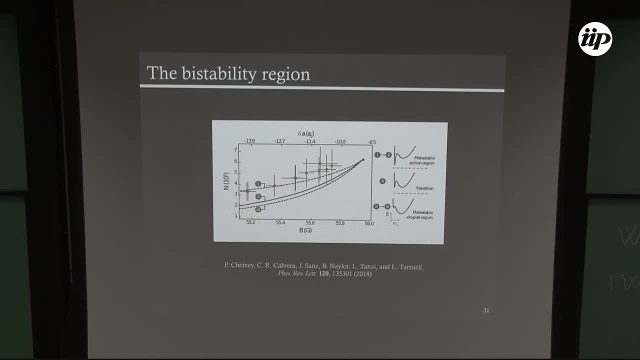 The ones I have explained just before. these are the bi-stable region. this black line from here is the transition where the two minimas, the soliton and the droplet, has the same energy. the top line is a meta-stable soliton, the bottom line will be a meta-stable. 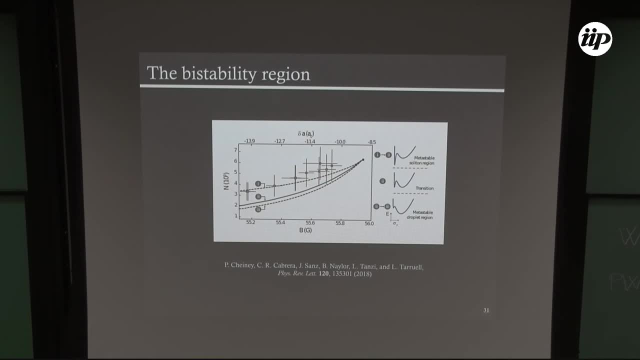 droplet and what we observe is that the fragmentation occurs on the top line, and this is because, in the experiment that we are doing, we start with a soliton that enters in this direction, so it follows the minimo, and then at some point this minimo becomes meta-stable. 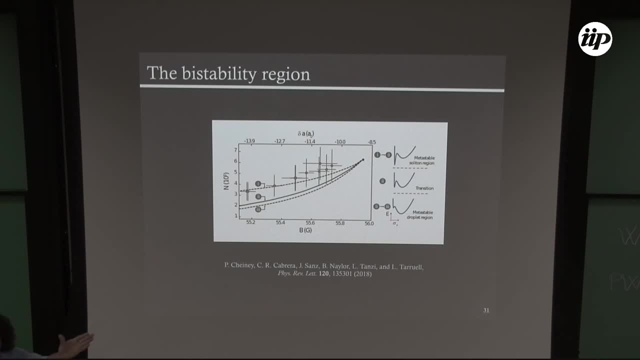 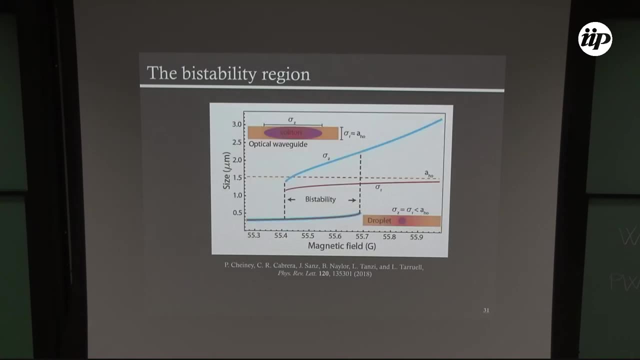 But still the minimo exists. so we just stay in the meta-stable minimo, but then at some point after this line, this minimo just disappears, and this is where we observe the fragmentation of the system. And again, this is what I was explaining before. 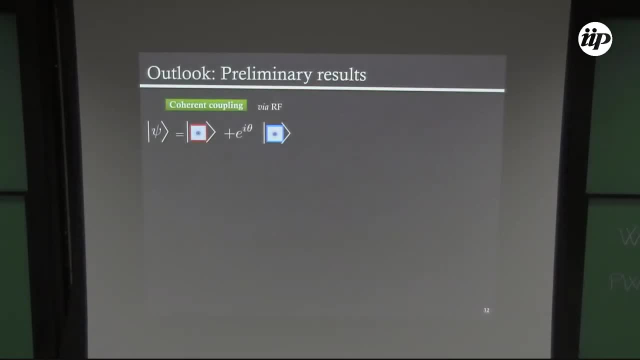 And with this I conclude. so this is what we have done so far at ICFO. then now we have upgraded our system and now we are studying a coherent coupling of these Bosse-Bosse mixtures. so what we are able to do is be a ref. 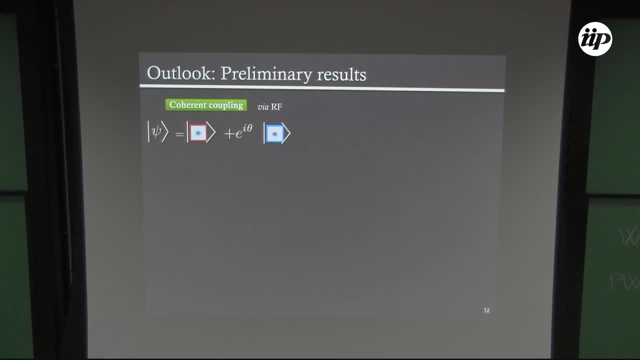 We are able to coherently couple the two components of the droplets. and the first experiment we have performed is that when we go to this dress state, the scattering between the particles is not just the normal scattering between each condensate, but it's 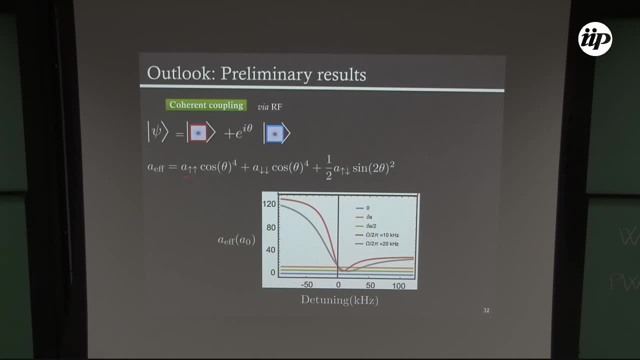 the scattering on the dress state picture of each dress state and in fact the effective scattering length of the system is given by the intra- and inter-species interaction and this value of theta that depends on the tuning of coupling between the two states. 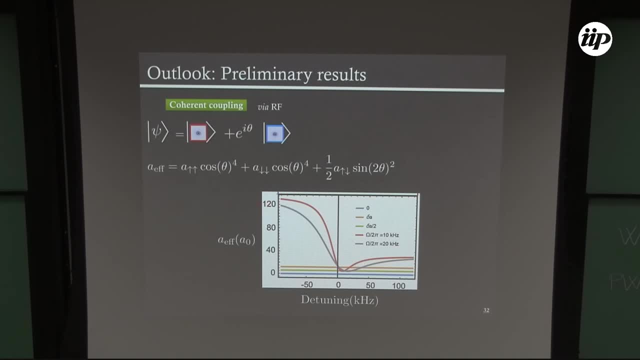 and the coupling strength. This is the way that, in principle, we can tune the scattering length it can go from I don't know like, for example, 120 to 40, that will be. 120, for example, will be. I up, up and 40. 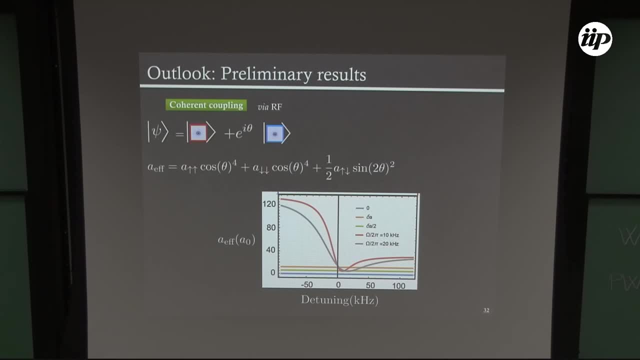 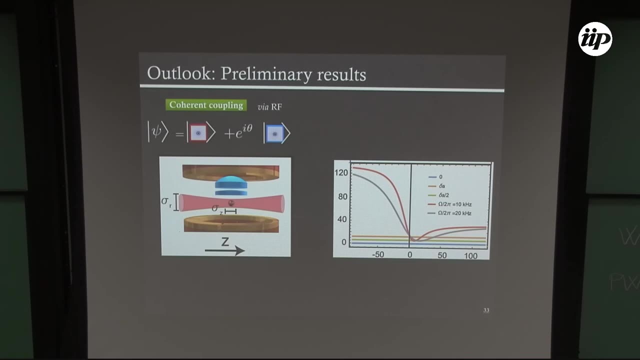 or 30 will be A down down, so we can see that we can control the scattering length in this way. What we have done, then, is we have started with a pretty simple experiment. so we have our optical waveguide, we have a Bosse-Einstein condensate. 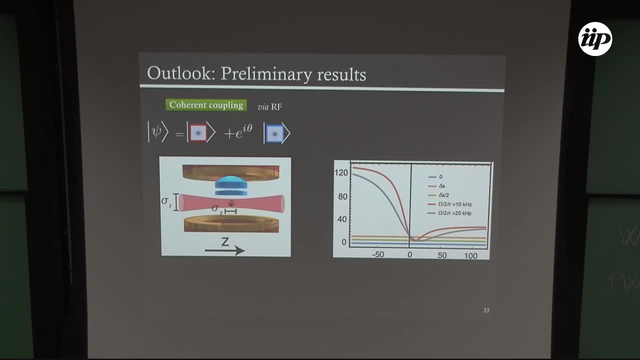 We do this: We couple Bosse-Einstein condensate, Bosse-Einstein condensate in this waveguide, and then we let the system to expand and with what we have observed, what I plot here is the width of the condensate as a function. 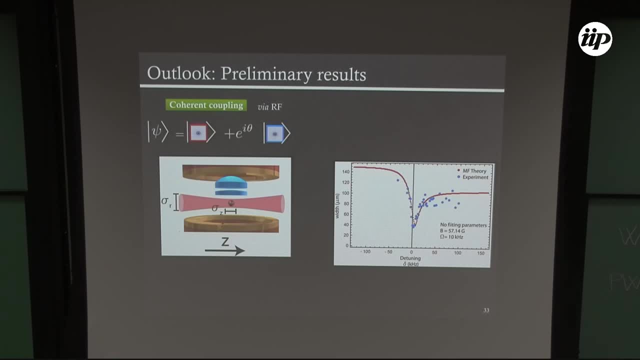 of, I mean for a given time, t and, as we know, depending on the interaction strength of the condensate, they will expand more or less and in fact this is the way that we can extract the scattering length of the system. and what I show here are the blue points where 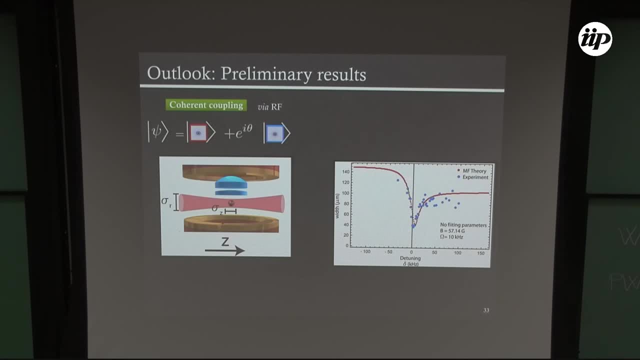 we can observe that, in fact, we are able to prepare this dress state. We are able to control as well the scattering length, and this is just some mill-fitting theory that I put on top. Some last experiment that we did as well is because we can tune the scattering length. 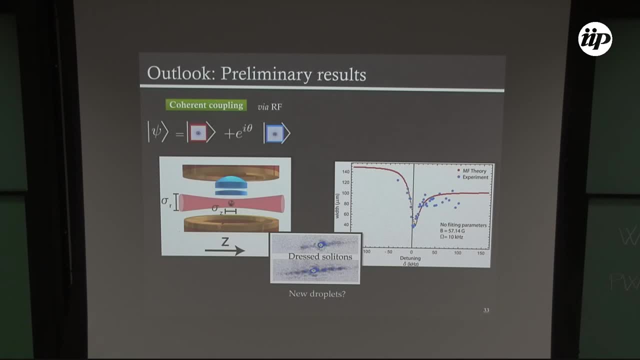 so now we go to a regime where, in fact, this effective scattering length can be zero or negative, and then we have seen as well the formation of these dress solid already, this optical wave. So now the question or the outlook that I want to give, is that we will start studying. 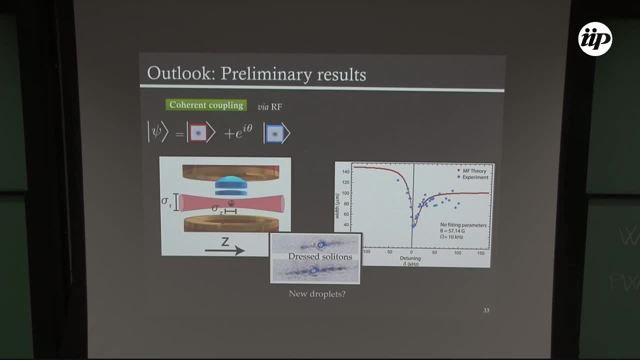 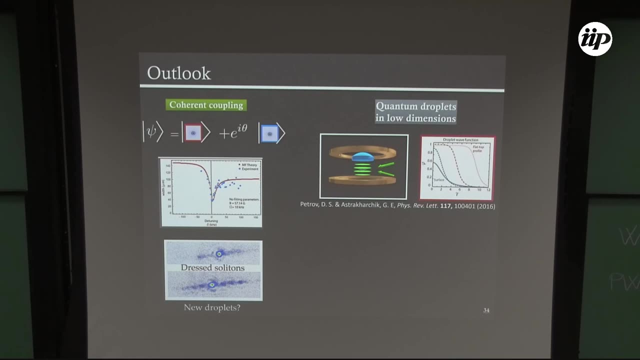 also new kind of droplets, Droplets that are coherently coupled. So other route that we are studying at DICFO is to go to low dimensions, either prepare droplets in 2D or in 1D dimensions, and with this I think I can conclude and I would like. 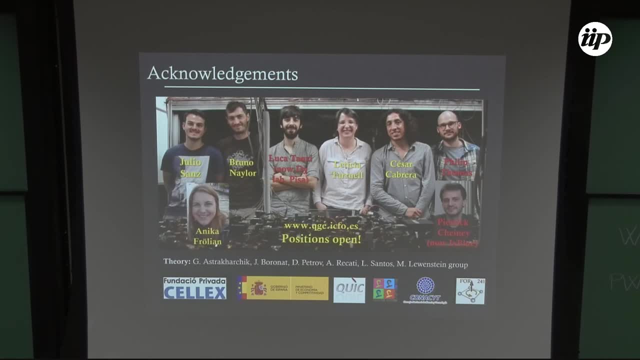 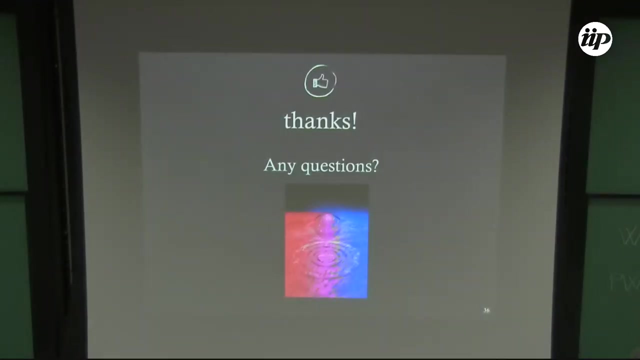 to thank my team and, in particular, Leticia Teruel, that unfortunately she's not here, but she really wanted to come And that's it, Thank you. Thank you very much. Thank you very much. Thank you very much, Cesar.